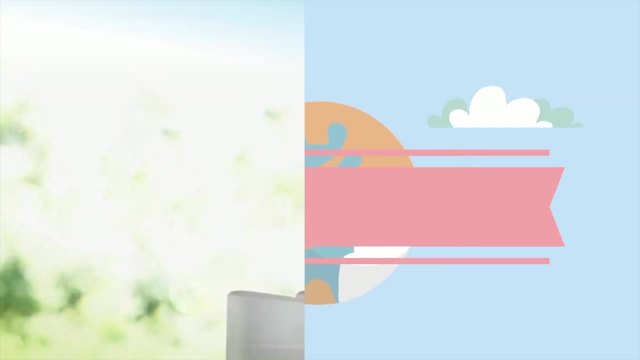 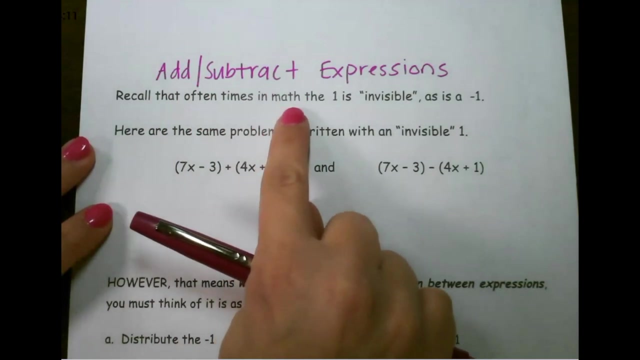 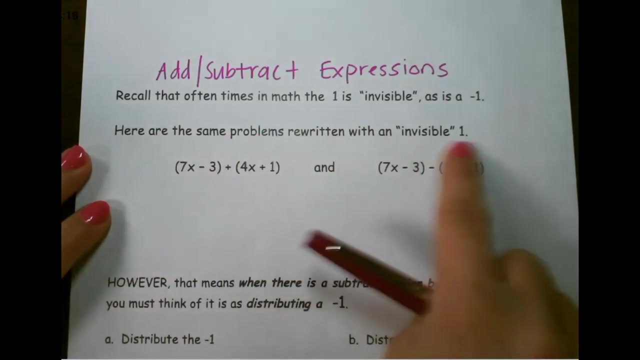 Adding and subtracting expressions. Remember that often times in math the 1 is invisible, as is a negative 1.. Here are the same problems, rewritten with an invisible 1.. So here we have a plus sign in the middle. Notice that there is no 1 here, so it's like an invisible. 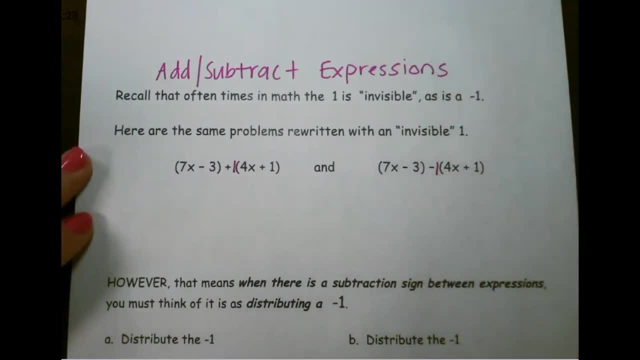 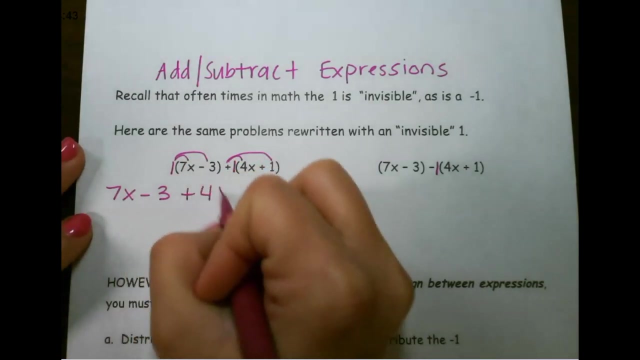 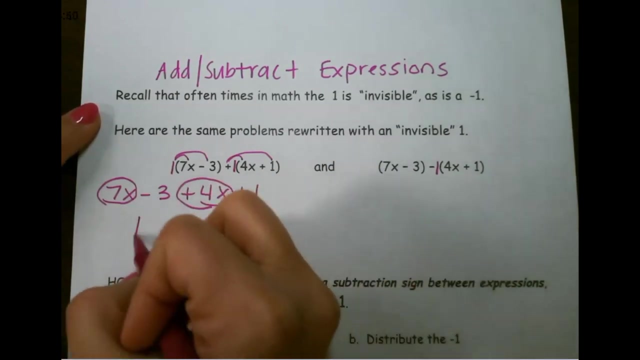 1, as well as over here. So with this first problem nothing changes, because if I were to distribute a positive 1 to everything on the inside of the parentheses, it would stay the same. So we simply just drop the parentheses From here. we combine like terms 7x and 4x. 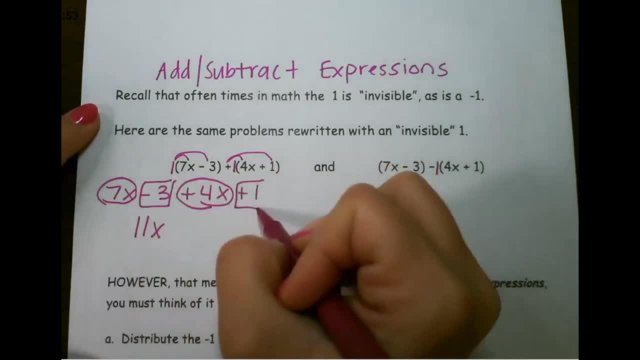 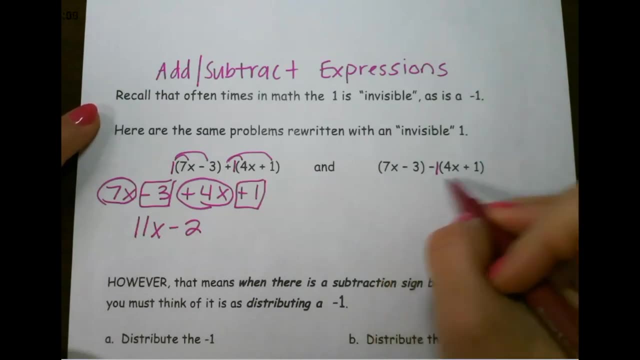 would give me 11x. Negative 3 and positive 1 would give me negative 2.. So that would be our answer for that one. But if we look at our second one, on our second expression, since there is a subtraction sign in the middle, we are distributing negative. 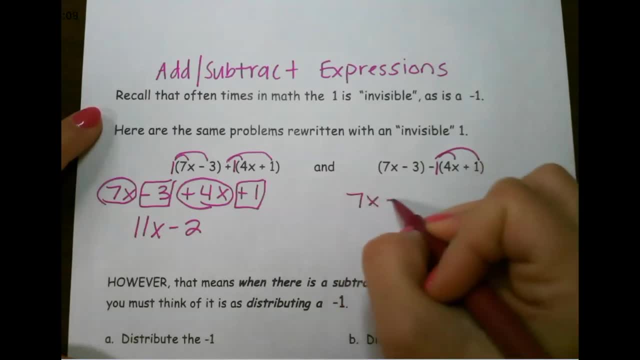 1 to everything inside the parentheses. So the first one stays the same, but the second one you flip the sign of everything in the parentheses, So this first term becomes negative 4x, and instead of plus 1, it would be minus 1.. Then we combine like terms. 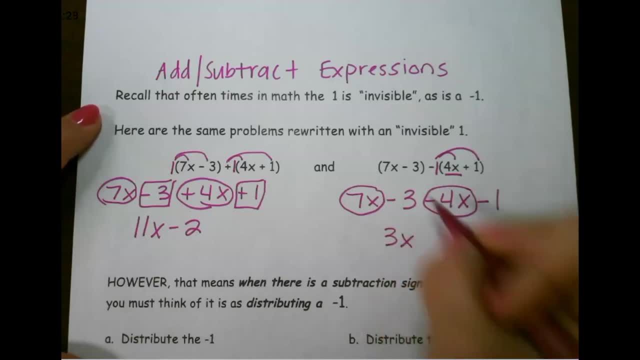 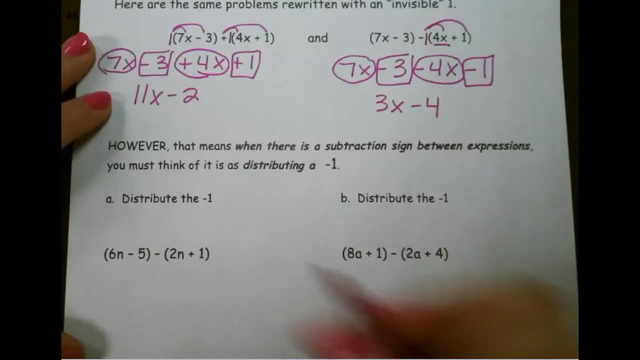 7x minus 4x is 3x and negative 3 and negative 1 would be negative 4.. On this next example, again, we have invisible 1s. This one is just positive 1, so it doesn't. 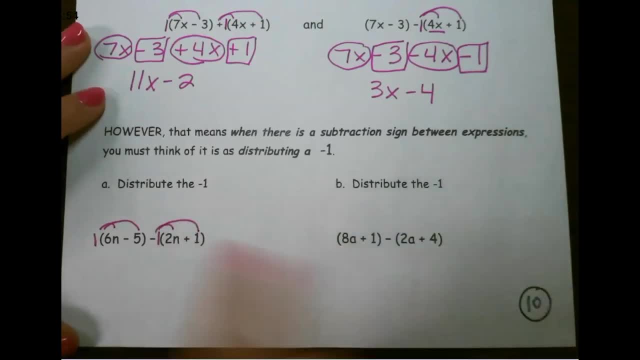 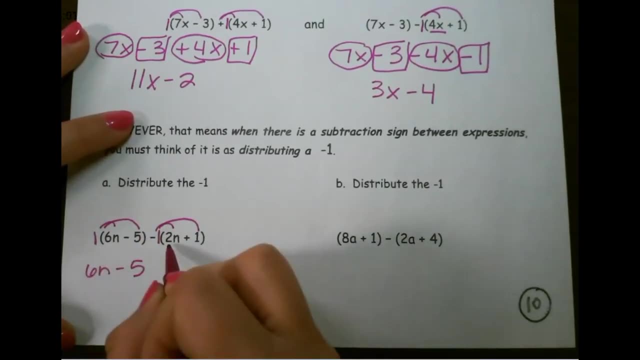 change anything and this one would be distributing negative 1.. So we change the sign of everything in the parentheses, So 6n minus 5. This becomes minus 2n minus 1.. Combine like terms, So 6n minus 2n would be 4n and negative. 5 minus 1 is negative 6.. 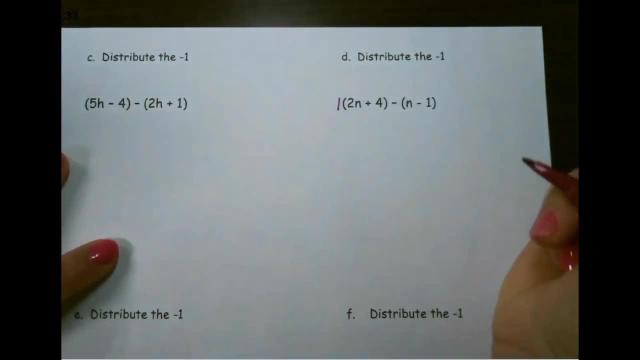 Let's look at this last example. So again it's just positive 1,, so that doesn't change anything about our first expression. But here we're distributing negative 1, which means everything on the inside needs to flip. So n is going to become negative, n and minus.